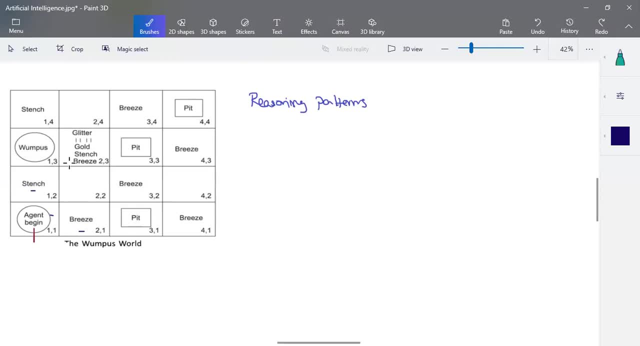 sensing of environment or conditions, whatever is available right now. based on that percept, we are going to take some actions out of it. Okay, so that is your usual agent based problems in all. So now the agent is going to enter into the cave in one comma one, and with that known fact, that one comma. 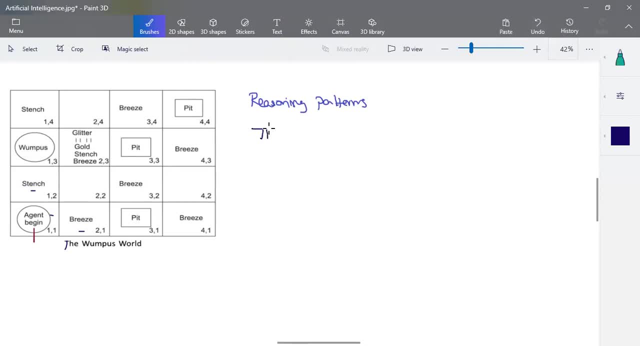 one is totally free, right, you don't have anything into it. so there is no breezy effect or there is no stingy smell And there is no pit or more. First, you have a lot of representation. you can use this representation for it. Okay, so with all this, we can proceed to the next step, since the death note is like: uh, there is no. 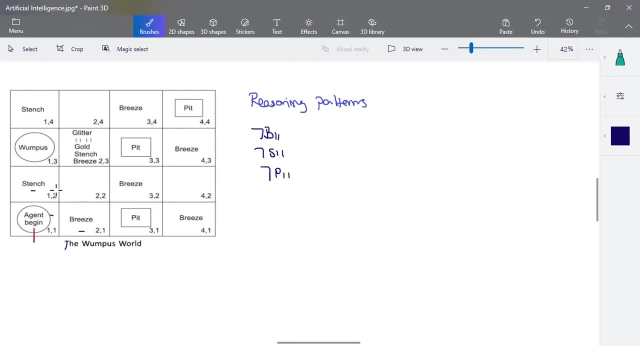 breeze. so there is no uh, no pit in the nearby rooms and there is no stingy smell, so you don't have any uh, or you don't have any pit in the uh, sorry, oomphers in the nearby room. so this can be represented like a rule. See, there is no breeze in one comma. one implies 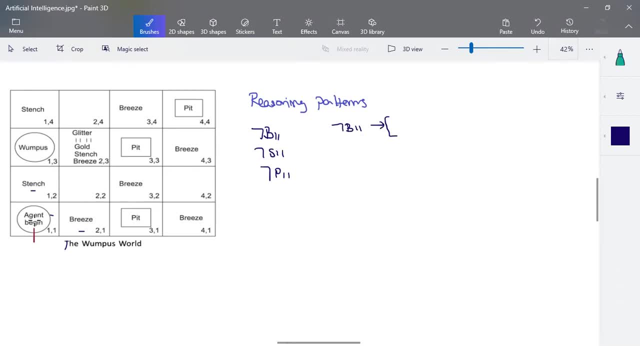 is no pit in the nearby room. so what is the nearby room for one comma one? One is one comma two and two comma one. So you can write it as there is no pit in one comma two and there is no pit in two comma one. We are going to use an and relationship. the reason is: there is no breeze. 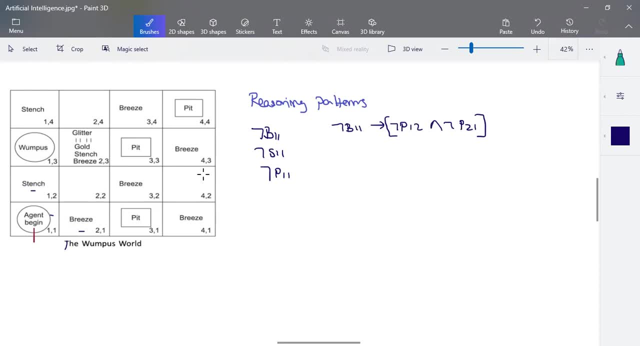 so surely both the adjacent rooms are not going to have a pit into it. okay, and there is toast and cheese, small, in 1 comma 1.. This implies there is no oomphers in the nearby room. 1 comma 2. and sorry, there is no oomphers. We can use this representation w for representing oomphers. 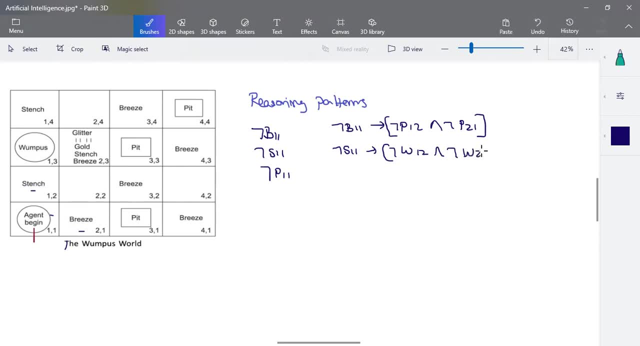 in 2 comma 1.. Okay, so this is how we are going to write the rules in the knowledge base. So when an agent enter into a room he will sense the current scenario, current enjoyment, whatever is the current perspective of the environment. that will be added as the rules in the knowledge. 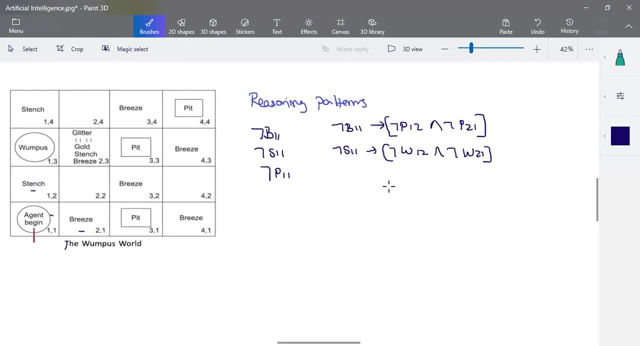 base. So each time when an agent tends to explore a room, he tends to derive some new rules out of it. Okay, so with this we can say that there is no breezy effect or a stenchy smell in room 1 comma 1.. So it is safe to enter into the room 1 comma 2 and 2 comma 1.. The reason is there is no pit. 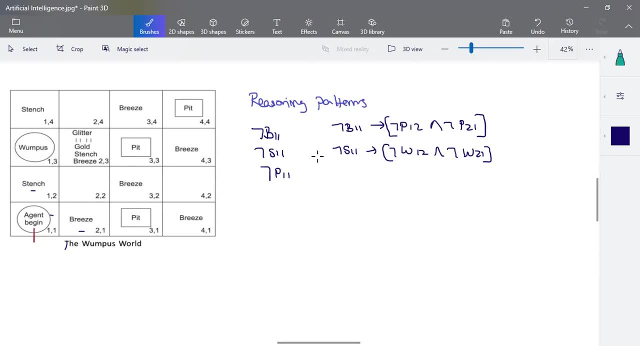 and there is no oomphers going to present in this place. Okay, to correlate these two rules. see this: there is no breeze in 1 comma 1 is proven, and this is a rule that if there is no breeze in 1 comma 1, then you don't have any pit in 1 comma 2 and 2 comma 1.. 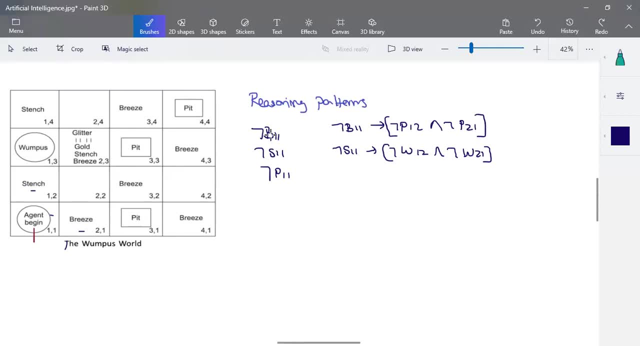 So this can be combined together and with that we can derive, like these two rules can be combined together and we can derive it, derive a new rule out of it, like combining these two. we can write it as there is no pit in 1 comma 2 and there is no pit in 2 comma 1.. So this kind of rule. 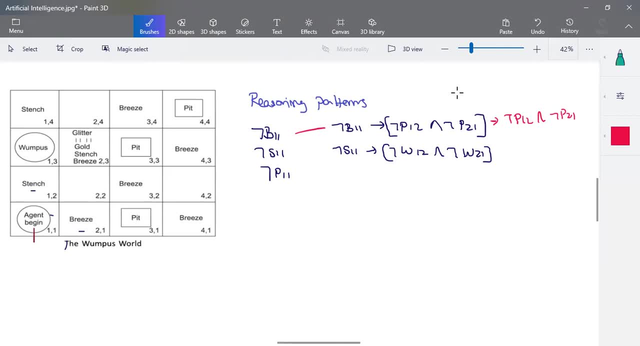 combination. right, this is called as Modus Podens rule. I'll tell you three rules, three basic rules that you usually follow. So one is Modus Podens. So it says that P implies Q, given P. these two are true. it says that Q is. 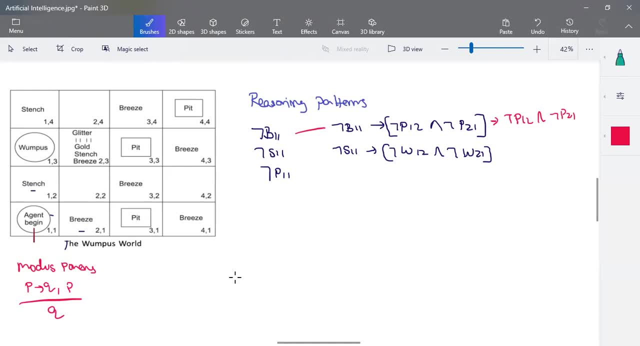 true. I usually convey this with an example like we can have this as an if-then-else statement implies actually says that it is an if-then-else statement. If it is raining, then street get wet. Whenever it is raining, then street get wet. 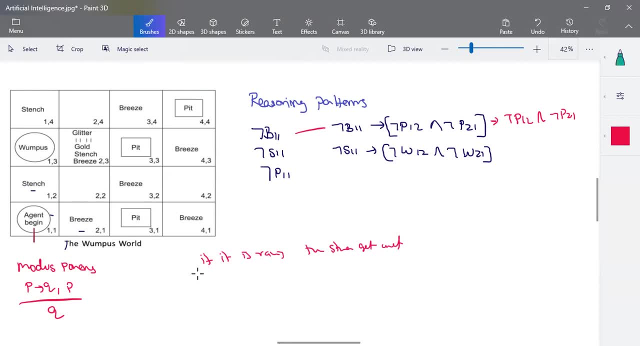 So this is a proven one. So that is how your implies is known and it is also known that, like, this is your P statement and this is your Q statement, Whenever it rains, the street will get wet. So this is a proven condition. it is going to be true for all when it is given as an implies. 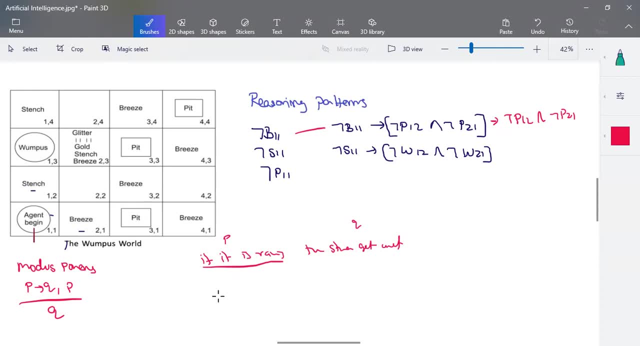 condition and given that it is raining now. So with that we can come to a justification that the street will get wet, So that you can relate it for a Modus Podens rule like another one is like this thing rule with a slight modification. 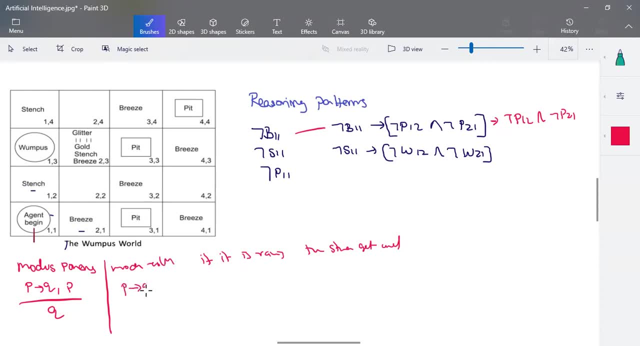 We call it as Modus Tolens rule. Modus Tolens is P, implies Q, negation P or Q is given. So whenever it is raining, the street get wet. and it is given that the street is not wet, So it means that this there is no rain in the place. Okay, so this is two main rules. 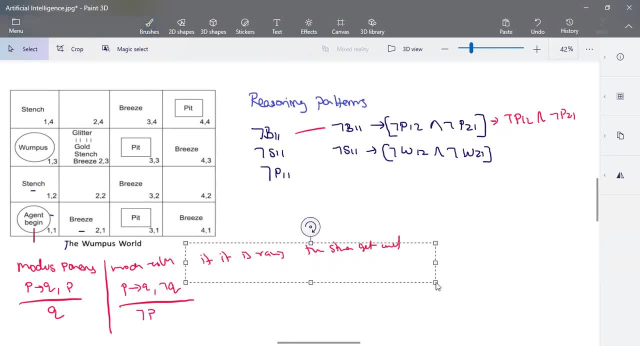 that you're going to use. and one more important rule is and elimination- See whenever you say that these two statements are true and when you combine, using that and connection- see here In the given example, it is known that, like using your Modus Podens rule, we can write it that there. 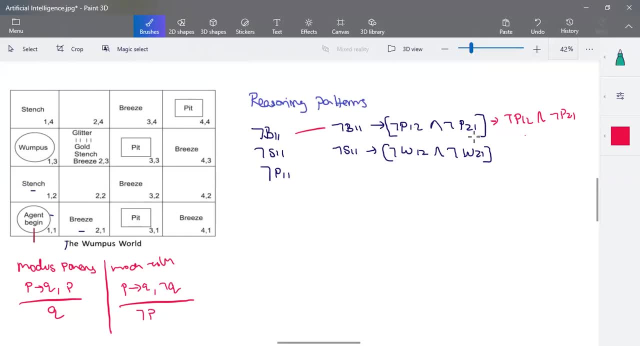 is no PIT in P 1 comma 2 and there is no PIT in 2 comma 1.. With that we can say that, like you can write it as no PIT in 1 comma 2, that is also true. No PIT in 2 comma 1, that is also true. So we can. 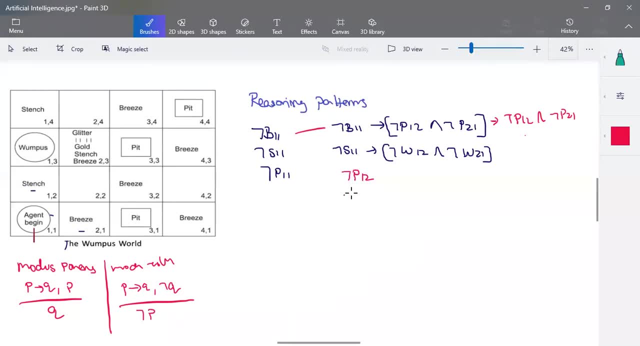 directly derive the rules, as there is no PIT in 1 comma 1 and there is no PIT in 2 comma 1.. So these two are proven one. Okay, so this is called and elimination, and elimination is something like when you have two rules combining, using and condition. it means that you can write a comma. 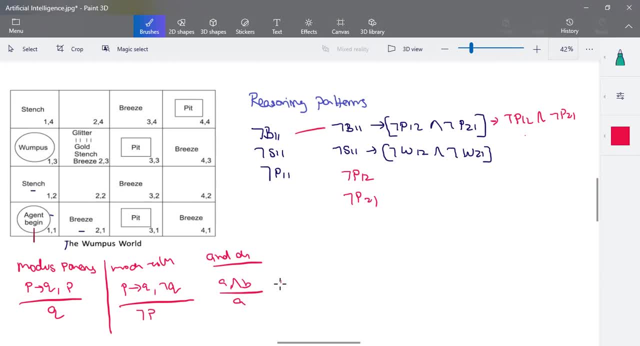 a and b. if it is taken to be true, it is a is true and b is true. You can write it as anything. this is your and elimination rule. Okay, so, using these rules, we are trying to find a pattern out of it. We are going to try to find a reasoning out of it, like in: 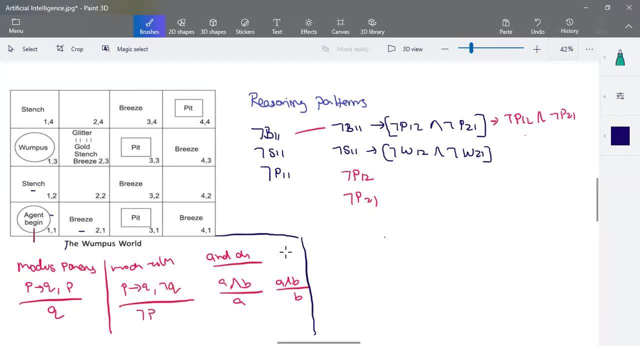 this example if I am trying to find a safer move next possible safer move. So after exploring this, 1 comma 1. You have two adjacent rooms. the agent can enter into either 1 comma 2 or 2 comma 1 and with the 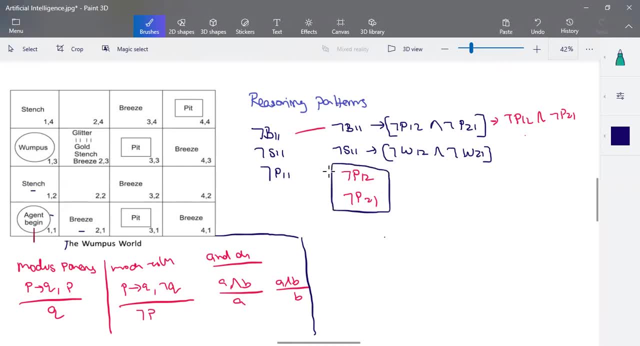 current scenarios, we can say that both the rooms are safe to enter. and now, when the agent want to explore this room, Okay, when the agent is exploring this room of 2 comma 1, there is a breezy effect in this room, 2 comma 1.. Okay, so it is known that there is a breeze in 2 comma 1. and when 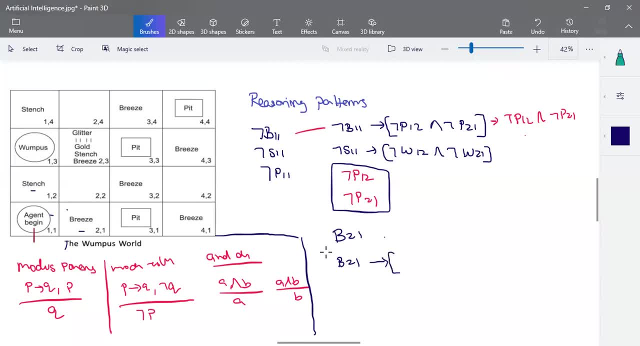 there is a breeze in 2 comma 1, this actually implies somewhere around this room you have a PIT. The rooms that are nearby PIT will have a breezy effect and when the breeze is detected it means that somewhere around the room we have a breezy effect. it might be either one. 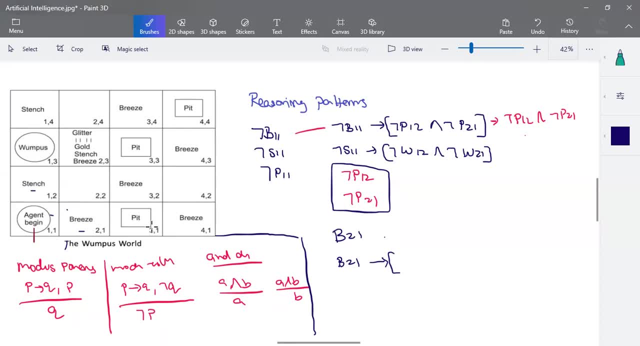 comma one, 2 comma two or three comma one, So you don't have any proper derivation of which room it is there. so this place we can use an AND connection so you may have a possibility or connection possibility of PIT in 1 comma 1 or there might be a possibility of PIT in 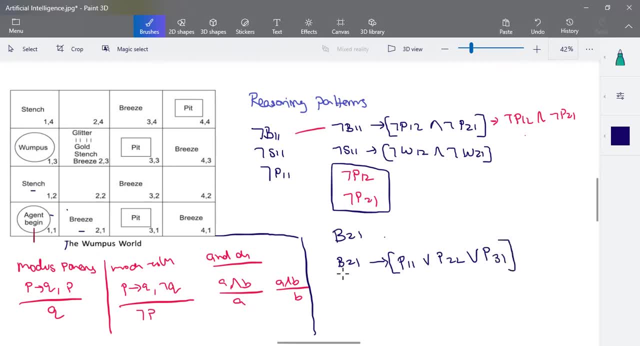 be a possibility of pit in 3 comma 1. okay, so using your modus ponens rule, you can write it as there is a pit in either p 1 comma 1 or p 2 comma 2 or pit in 3 comma 1. okay, so this you can write it. 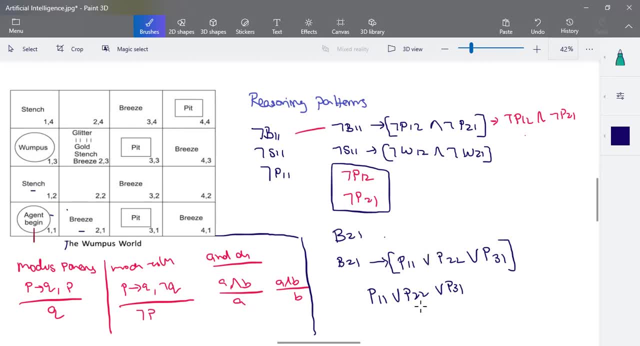 using your modus ponens rule, but with this we cannot have a proper justification of which room to enter next. okay, so agent cannot take a risk on entering into a room that consists of pit. so either 2 comma 2 or 3 comma 1 will have a pit, since it is already given that there is no pit in. 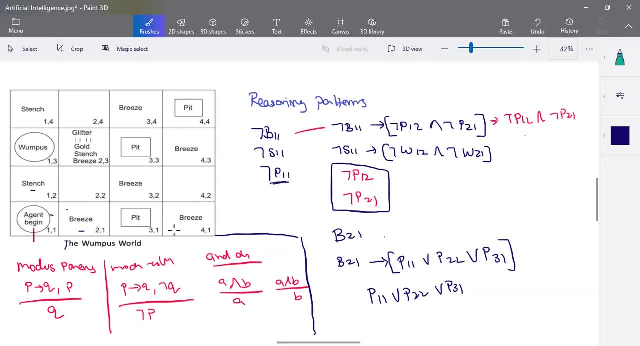 1 comma 1. okay, so you have another two possibilities. we cannot take a risk in this, so we can. what we can do now. the agent can take the next possible room over here. okay, so we have already decided that 2 comma 1 is safe and we have entered into the room now. the next possible safer room is 1. 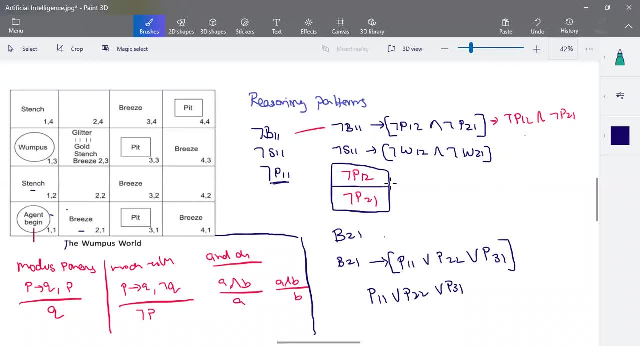 comma 2, so the agent when he is entering into this 1 comma 2, i'll take another color. i don't have space here. you I'll write it here. when an agent explores this 1 comma 2, it has a stingy smell, but since we are, 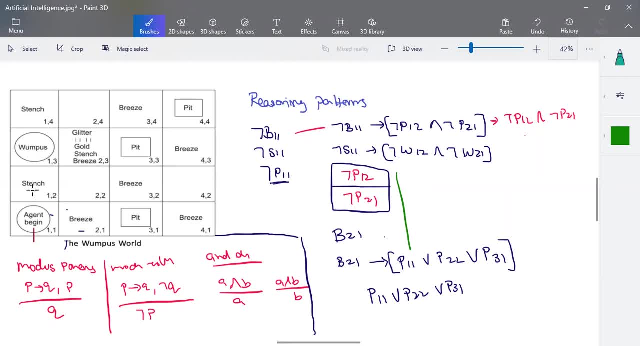 just focusing on the rooms that consist of pit alone. there is no breeze in the space. okay, so there is no breeze in this? 1 comma 2. so no breeze in 1 comma 2. what does it denotes? it denotes that there is no pit in the nearby room. so what are the rooms that are near to this room? 1 comma 1. 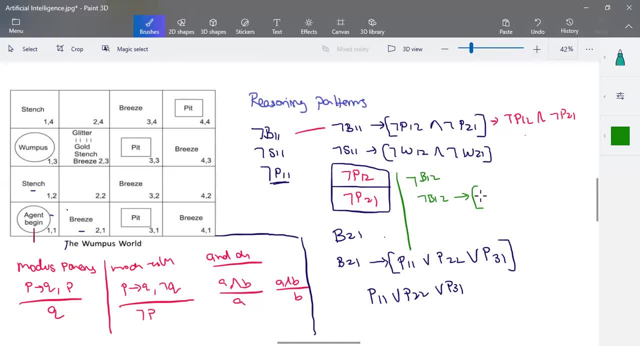 2 comma 2 and 1 comma 3, so we can write the rules as there is no pit in 1 comma 1 and there is no pit in 2 comma 2 and there is no pit in 1 comma 3. okay, using modus ponens. 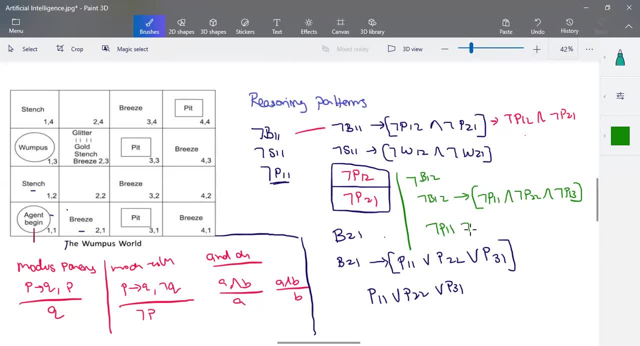 true, we can write it, as there is no pit in 1 comma 1, there is no pit in and there is no pit in 2 comma 2 and there is no pit in 1 comma 3, so all these things are derived. now what you're going to do. 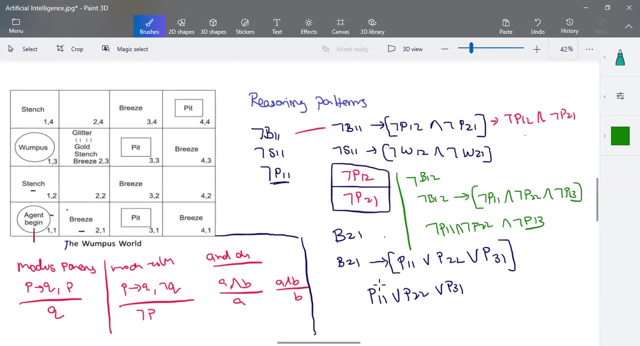 next. now, combining these rules, we can say that you have p 1 comma 1. a pit will be either in 1 comma 1, but pit in 1 comma 1 is not there. okay, by combining that there is no pit in 1 comma 1, we can write that you have a possibility of pit in either 2. 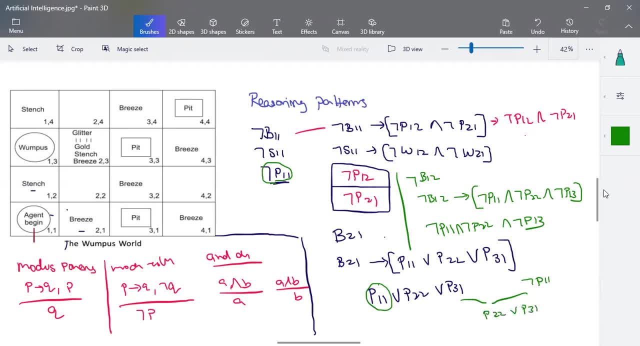 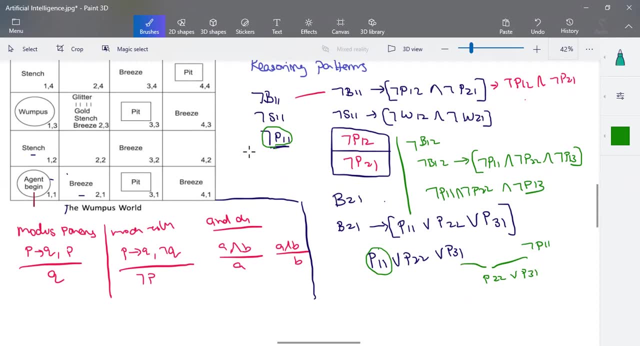 comma 2 or p 3 comma 1. okay, I hope you understand this, since there will be a possibility of pit in either 1 comma 1, 2 comma 2 or 3 comma 1, and we already know that there is no pit in 1 comma 1. 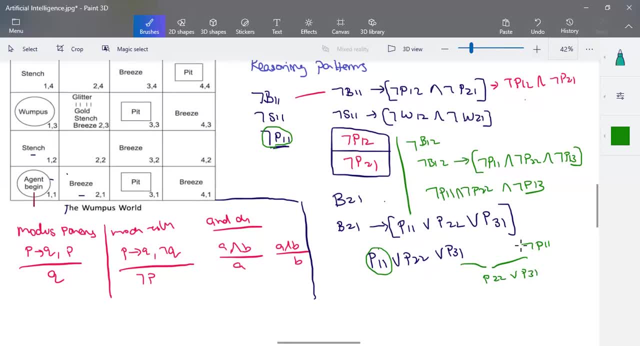 so with that we can derive either the pit will be in 2 comma 2 or 3 comma 1 and using this rule, when you use an and elimination place, there is no pit in 2 comma 2 is also, given there is no pit in 2 comma 2, by combining these two we can write it as there is a pit in 3 comma 1. 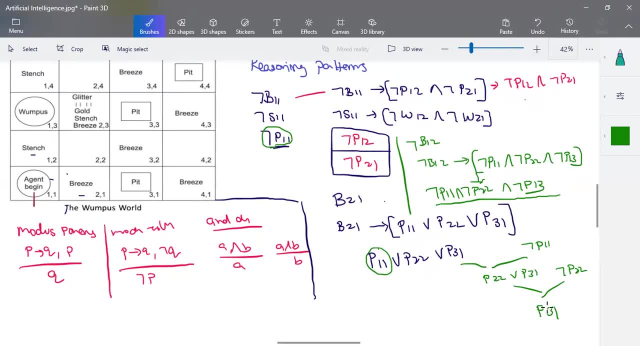 and you don't have any other possible rules that actually defines whether the pit is there or not. so with that we can prove that there is a pit in 3 comma 1. okay, so this is how we combine the rules: that derives or derived in a particular place we put: 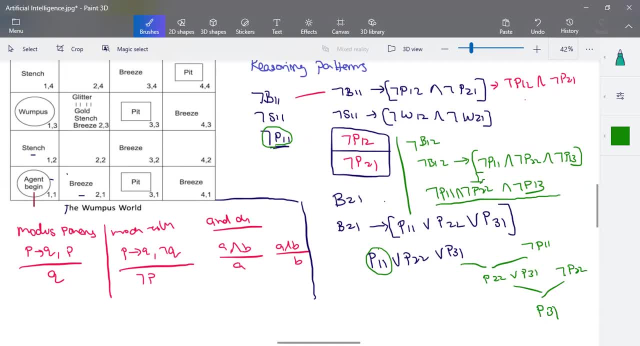 our knowledge base and we club two or three rules together to find a derivation out of it. okay, so this is how a reasoning pattern occur and when you want to find a resolution for any of the rules, like when you want to justify that there is a pit in 3 comma 1. okay, if it is given. 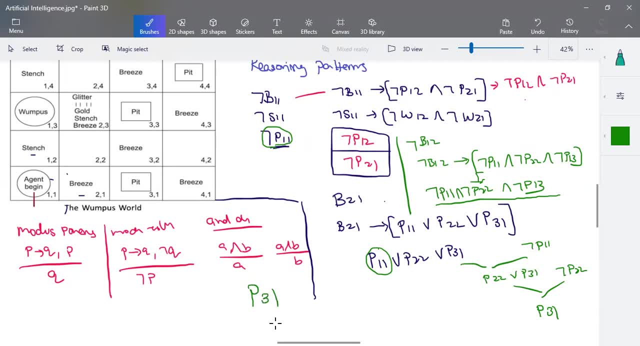 that when a goal is given that we have to find the pit in 3 comma 1, what we usually do, we take the negation of it and add it to the existing database. okay, so we take this as an resolution, like negation of p, 1 comma 1, and we take the negation of it and add it to the existing database. 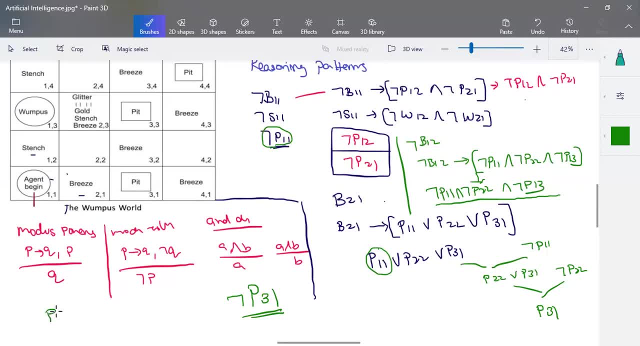 comma 3 is taken here, since my goal is to find there is a pit in 3 comma 1. so what we usually do, we take that, the reverse of it, negation of p, 3 comma 1, and we convert all the rules into a. 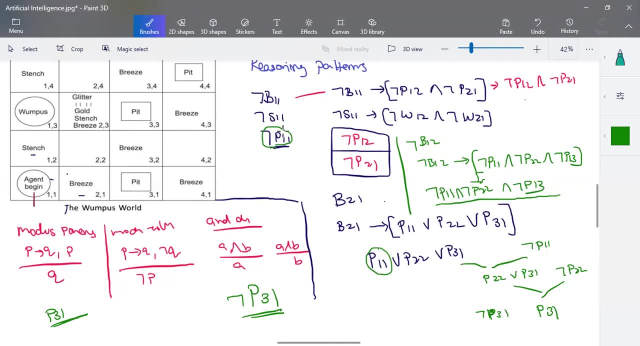 conjecture normal form. like all these rules that we have added right, these are all unconnected. so it is true that there is no grease in 1 comma 1. it is true that there is no stinky smell in 1 comma 1. so whenever an agent is exploring the rule, uh, exploring the rule, uh, exploring the rule. 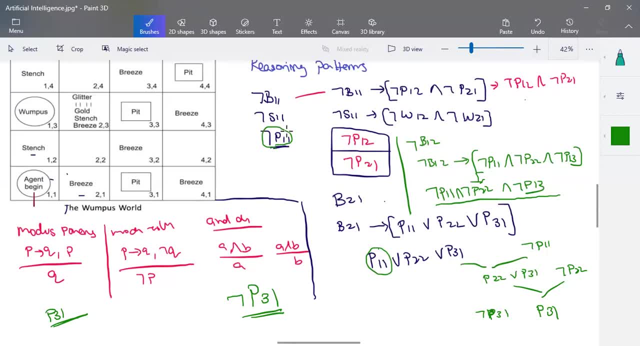 each and every room. all the rules that are generated are true. okay, so that actually means everything is true. it is all connected using a conjunction. it is in conjecture normal form. we have to use: okay, and we add this negation of the rule. convert all the rules into conjecture normal.